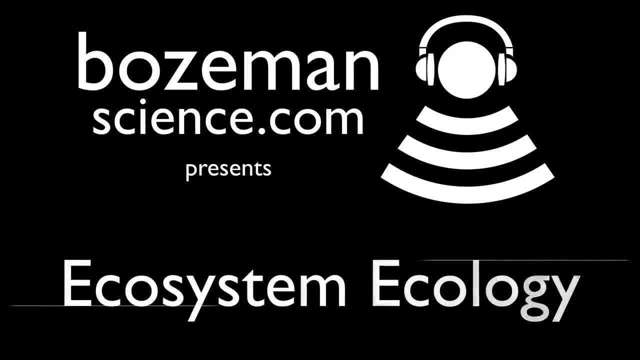 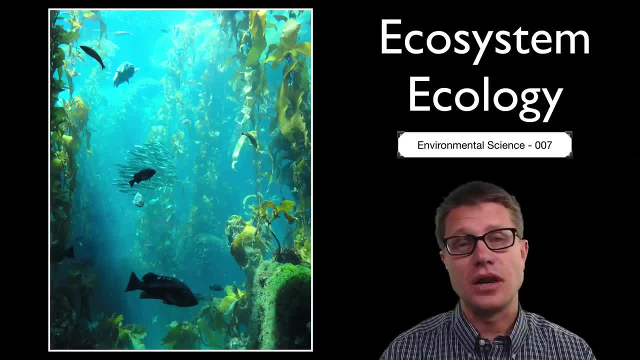 Hi, It's Mr Andersen, and this is environmental science, video 7. It is on ecosystem ecology. Ecosystems are large areas on our planet that contain both living and non-living material. A great example could be these giant kelp forests. The kelp are producers, So they are. 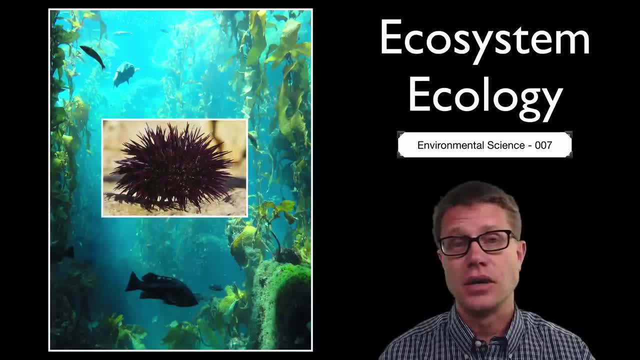 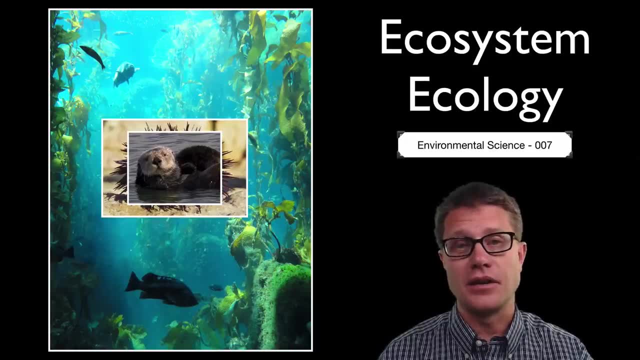 taking energy from the sun and converting that into food which is eaten by herbivores like this sea urchin, which, in turn, are eaten by carnivores like this sea otter. Now, the problem with the sea otter is, if it dies due to hunting or predation, then the sea 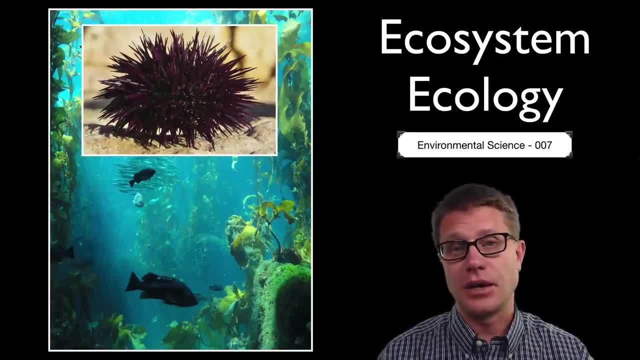 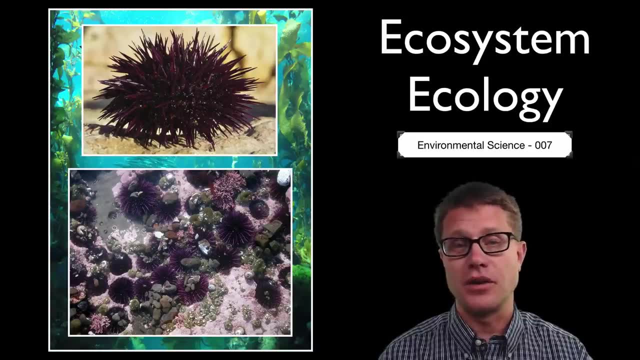 urchin populations will take off. Sea urchins feed on kelp by trimming the bottom, and sometimes the kelp will simply float away, And so if you have too many sea urchins, you get what are called urchin barrens, where there are no kelp and therefore the whole ecosystem. 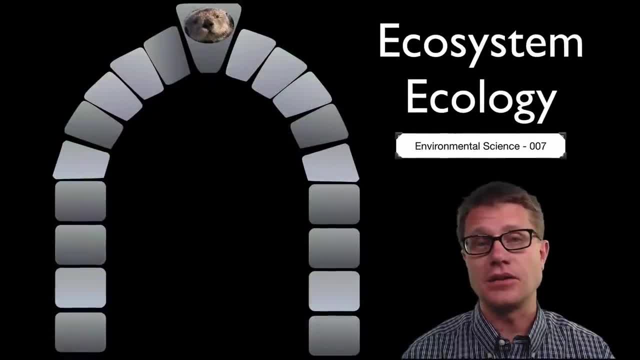 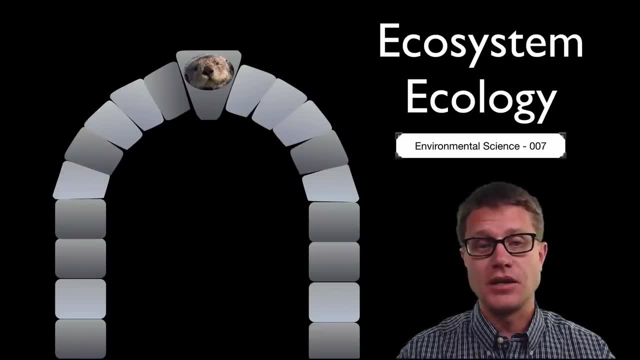 kind of folds in on itself, And so we like to think of the otter as a keystone species. Just like on this arch, this keystone at the top holds everything else in place. You can think of each of these stones now as a different species. If we remove that keystone species, then the whole thing folds. 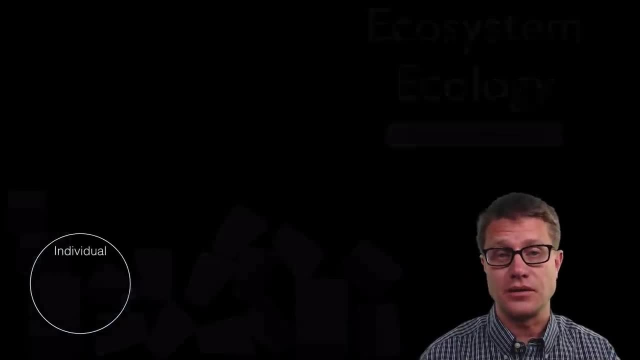 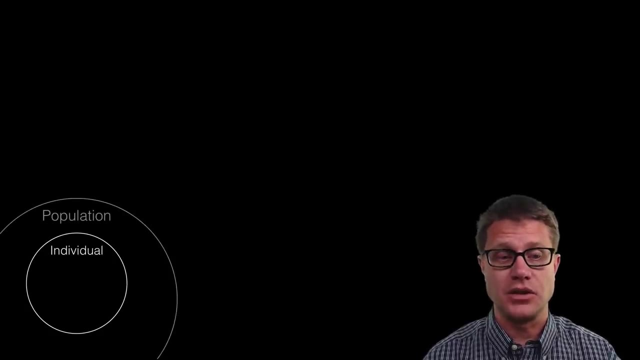 in on itself. In other words, some species are actually more important than others. Before we get to ecosystems, we should understand how life is organized. From the very small one individual. for example, sea urchin is part of what is called a population, or all. 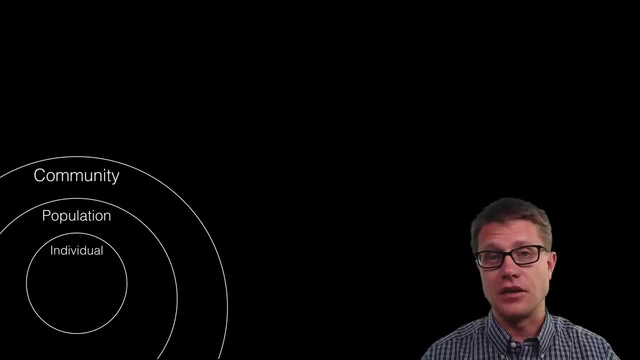 the sea urchins in an area. We then take all the populations together. That is a community. We then add the non-living material, That is an ecosystem. And then we even have larger areas, which are called the biomes. What is larger than the biomes? That is going to be the biosphere. It is going to be our. 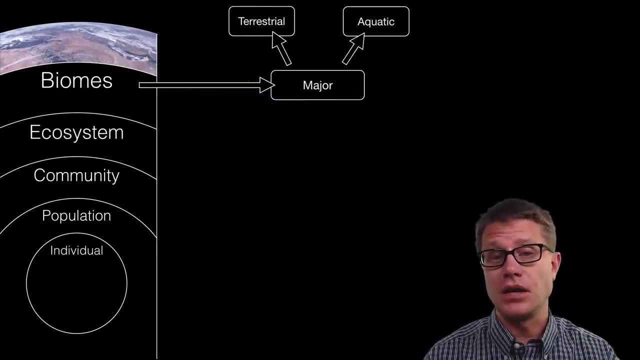 planet, And so, before we get to ecosystems, we will start by studying the major biomes, both terrestrial or land based, and aquatic, those in the land. We will then move on to the interactions at the ecosystem level. So that is going to be all of the producers and 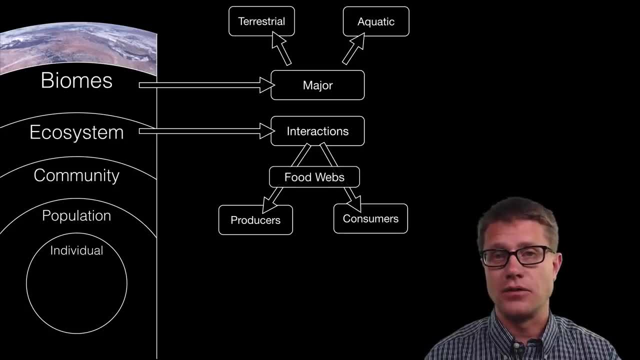 consumers interacting. A good way to study that is going to be with their food webs. We are also going to add abiotic or non-living material. We will then jump to individuals and the role of a niche. That is going to be the job. That is going to be the job That. 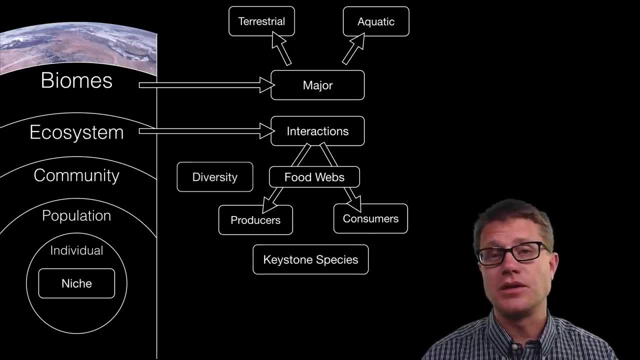 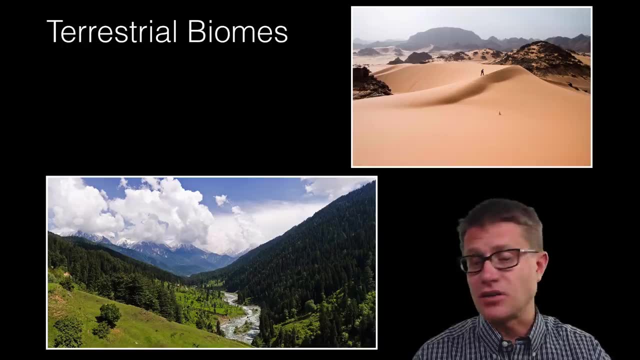 is an individual has. We will then move to the importance of keystone species diversity, and then, finally, edge effects and keeping that ecosystem healthy. And so let's start with terrestrial biomes. A desert could be an example, one A forest, a boreal forest. 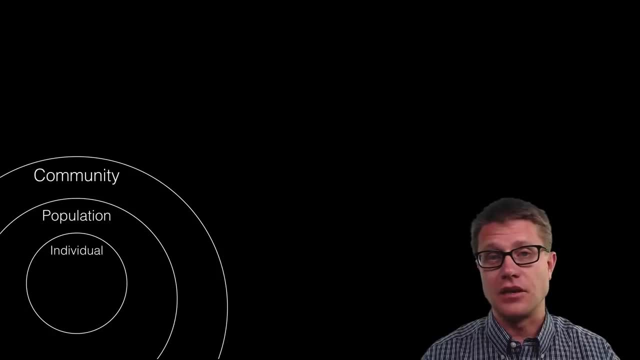 the sea urchins in an area. We then take all the populations together. That is a community. We then add the non-living material, That is an ecosystem. And then we even have larger areas, which are called the biomes. What is larger than the biomes? That is going to be the biosphere. It is going to be our. 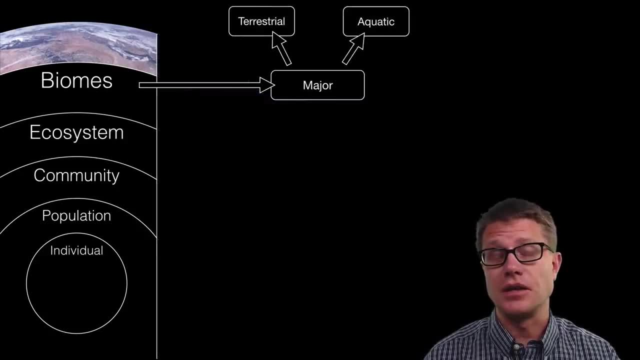 planet, And so, before we get to ecosystems, we will start by studying the major biomes, Both terrestrial or land based, and aquatic, Those in the land. We will then move on to the interactions at the ecosystem level. So that is going to be all of the producers and 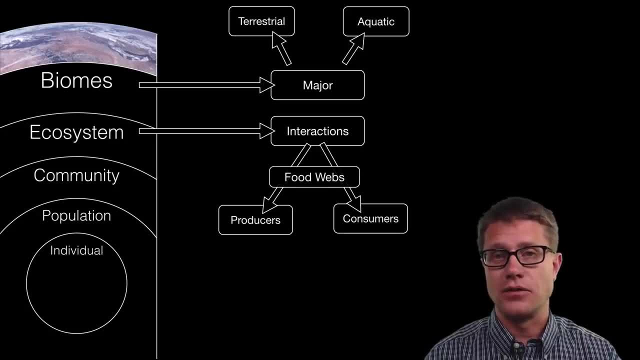 consumers interacting. A good way to study that is going to be with their food webs. We are also going to add abiotic or non-living material. We will then jump to individuals and the role of a niche or a niche. That is going to be the job The market is going to. 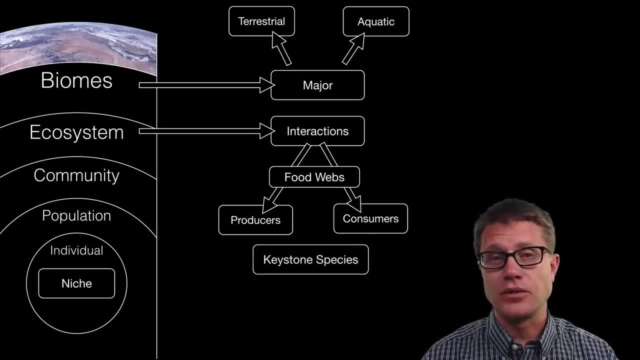 be the job. We are going to study the biomes. It is going to be the biodiversity that we are, that an individual has. We will then move to the importance of keystone species diversity And then, finally, edge effects and keeping that ecosystem healthy. And so let's start. 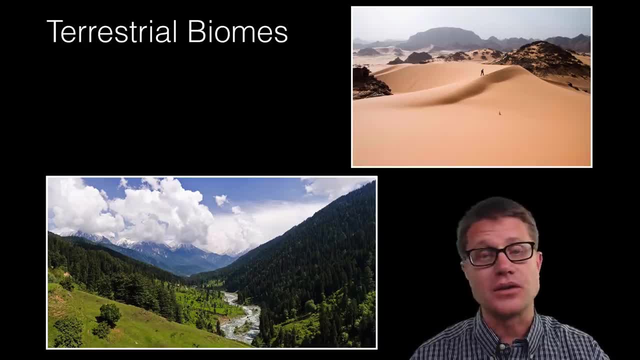 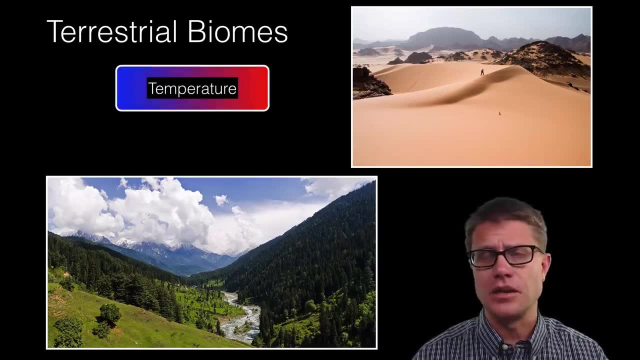 with terrestrial biomes. A desert could be an example, one A forest, a boreal forest, could be an example. Now, there is really only two properties that determine what biome we are going to have. That is going to be the temperature. average temperature and the average. 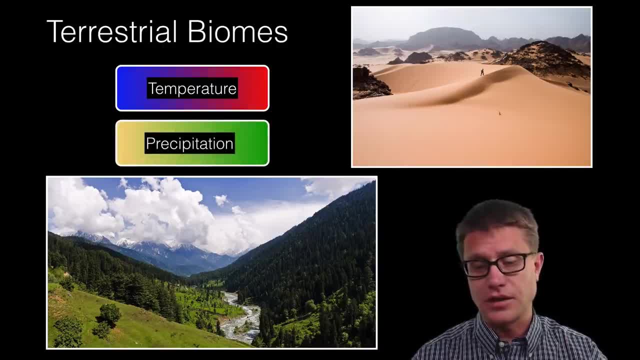 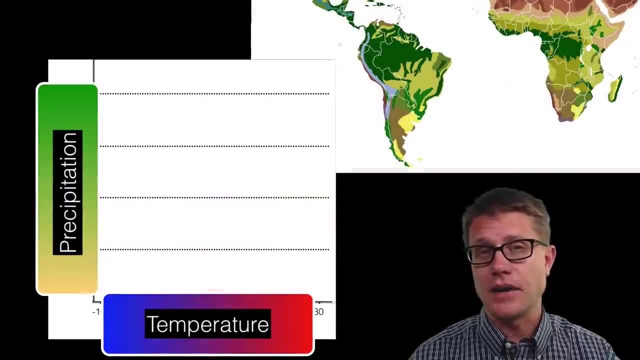 precipitation. So you could be given a map and just told what is the average temperature and precipitation And you could make a pretty good guess as to what the biome is going to look like. And so if we graph those on a graph where we have precipitation on the y, so that 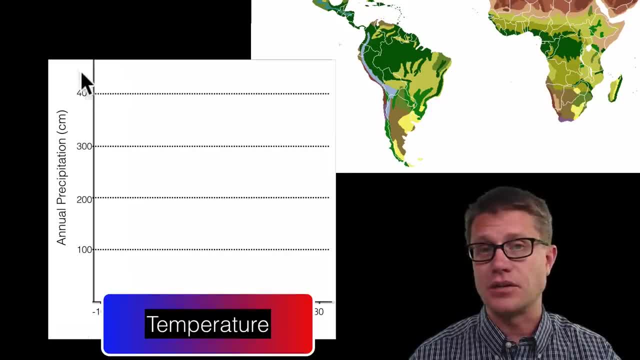 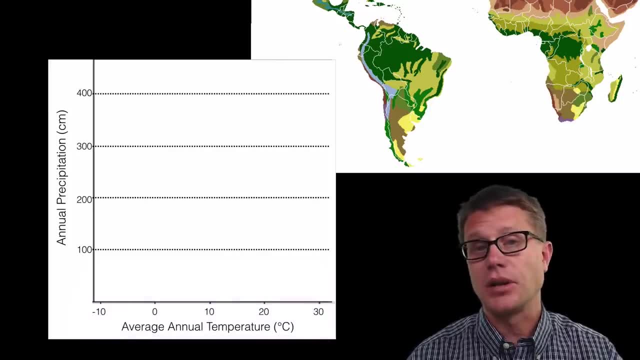 is going to be the amount of annual precipitation, from 0 to 400 centimeters a year. And then we look at temperature: from the very cold on the left- negative 10 degrees Celsius as an average, up to 30 plus degrees Celsius, You could kind of guess as to what biome are. 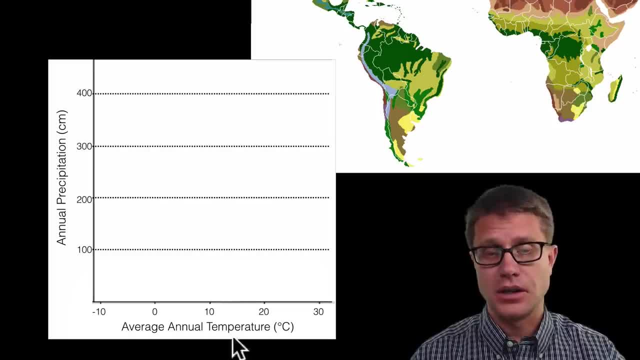 we going to find where it is really really hot and where it is really really moist. You could even point to it on our biome map. That is going to be the tropical rainforest, And so what you can do on this map is just read precipitation. 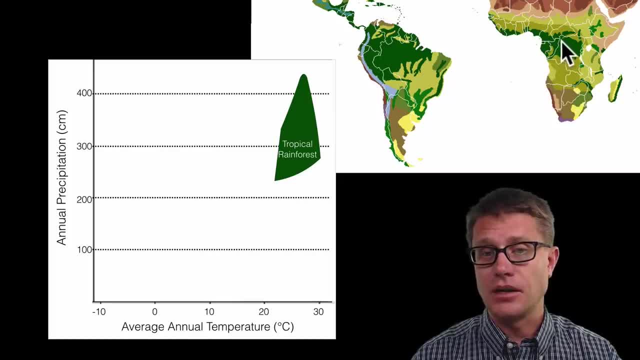 temperature. That tells you the biome. If we were to go in Africa right here and then move to an area where it is still hot but we have less precipitation, that is going to be a tropical forest or savanna- You are probably familiar with that. If we keep moving, 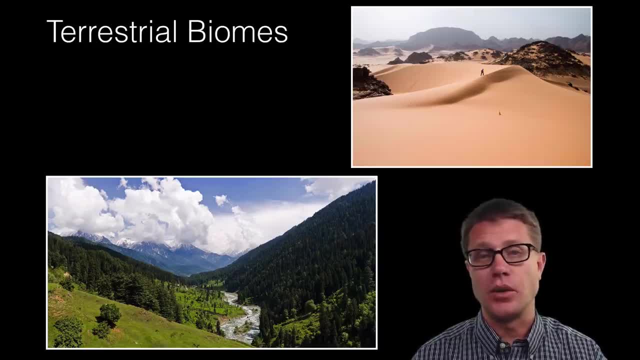 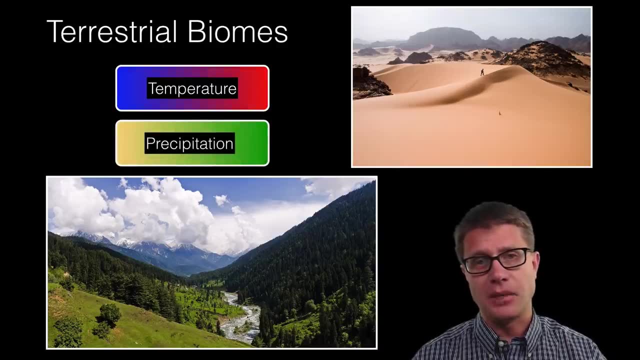 could be an example. Now there is really only two properties that determine what biome we are going to have. That is going to be the temperature: average temperature and the average precipitation. So you could be given a map and just told what is the average temperature. 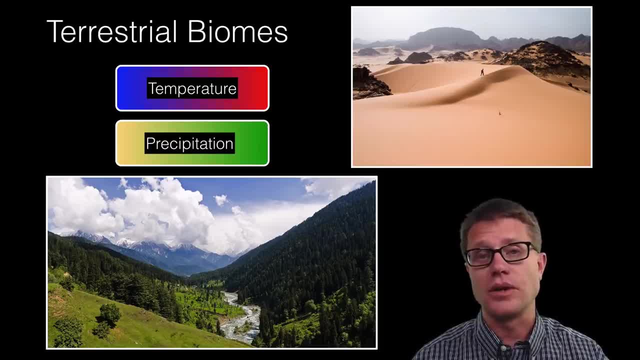 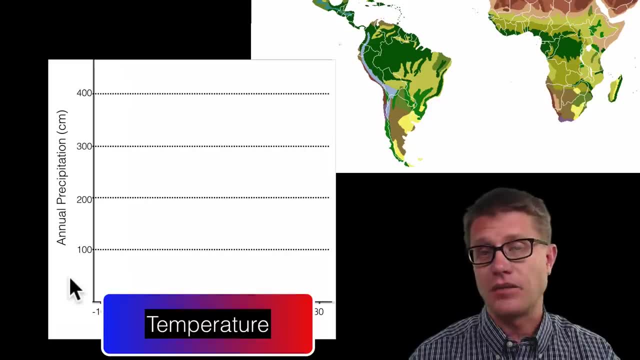 and precipitation And you could make a pretty good guess as to what it is. And then you could guess as to what the biome is going to look like. And so if we graph those on a graph where we have precipitation on the Y, so that is going to be the amount of annual. 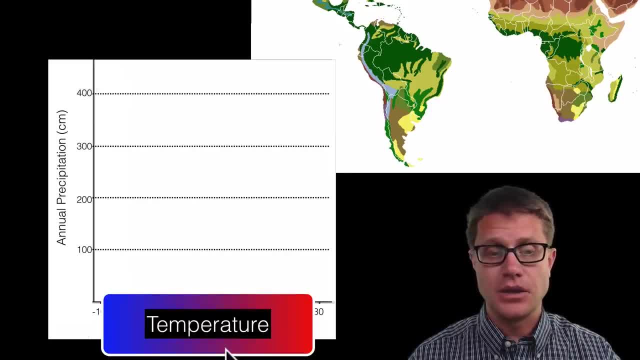 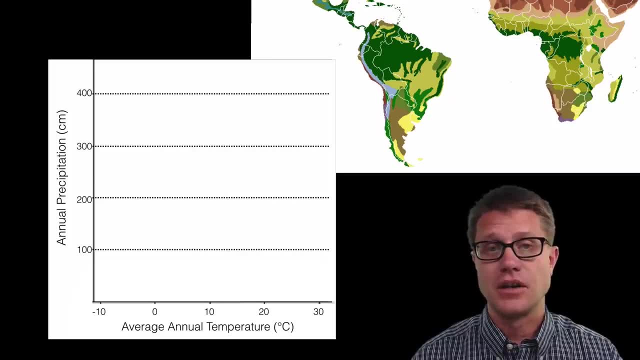 precipitation from 0 to 400 centimeters a year. And then we look at temperature, from the very cold on the left- negative 10 degrees Celsius as an average- up to 30 plus degrees Celsius. You could kind of guess as to what biome are we going to find where it is really? 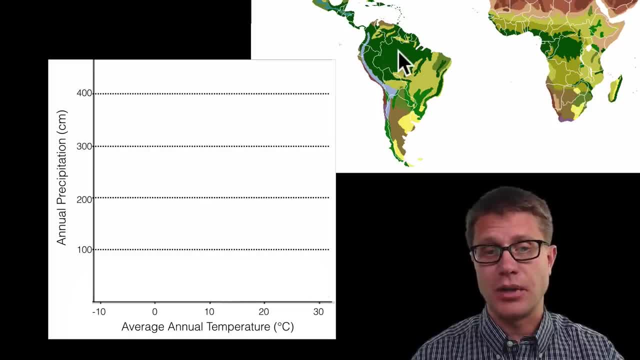 really hot and where it is really really moist. You could even point to it on our biome map. That is going to be the tropical rainforest, And so what you can do on this map is just read precipitation temperature. That tells you the biome. If we were to go in Africa. 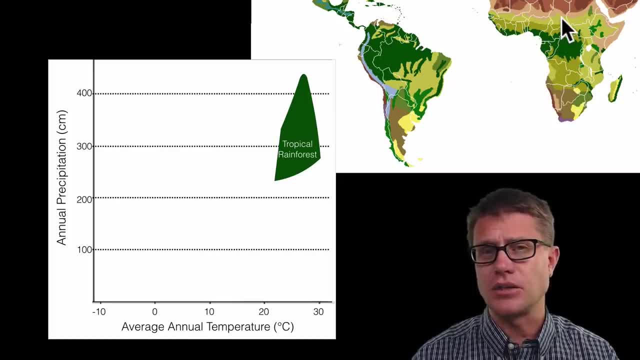 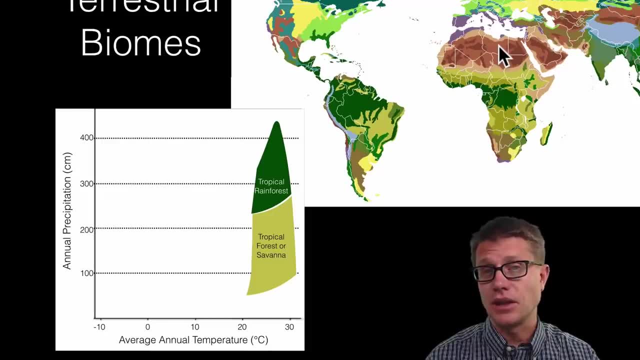 right here and then move to an area where it is still hot but we have less precipitation. that is going to be a tropical forest or savanna. You are probably familiar with that. If we keep moving up so we have even less precipitation, then we are going to get into a subtropical. 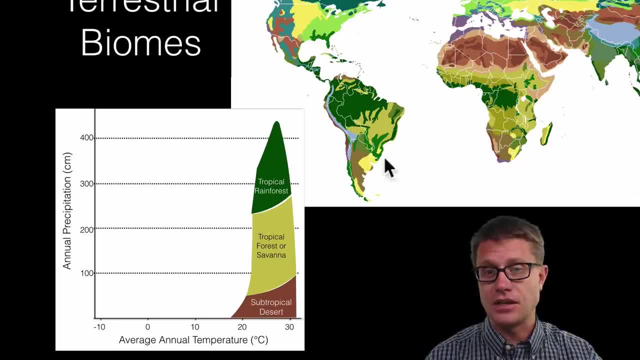 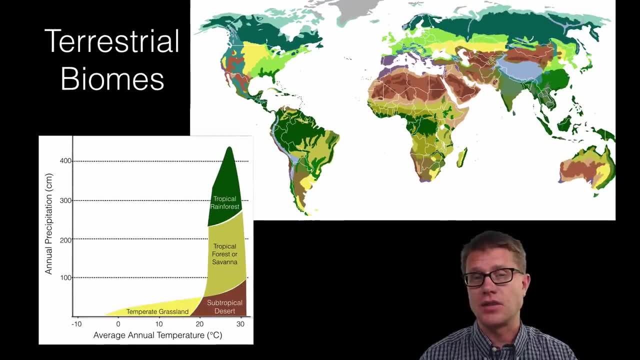 desert, And you can see those at this latitude and at this latitude right here. If we keep going across from Africa- though, let's go up here- we are then going to have temperate grasslands. Sometimes we have temperate deserts. You could. 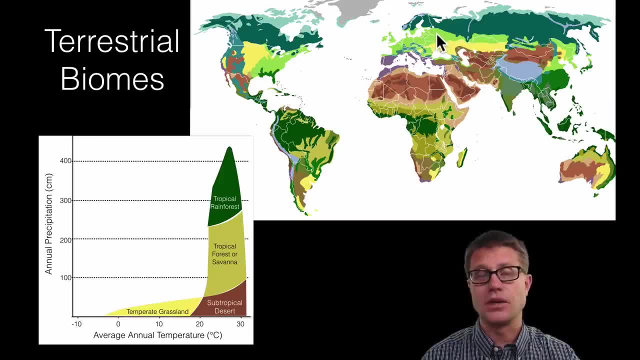 see that we have a lot of those in the Midwest of the United States. If we keep going then we are going to get to temperate seasonal forests. If we keep going then we go to the boreal or northern forests And then we eventually get to the tundra. So these are the major 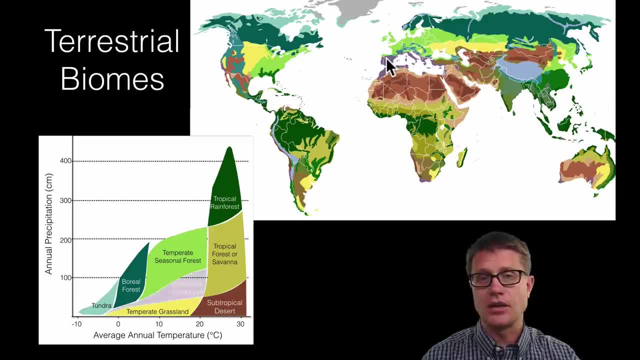 biomes. We could fill in a couple of other ones. So right here in the Mediterranean we are going to have woodland shrublands. We would have that over in California as well, And then, if we go up here, we will have these temperate rainforests where it is cooler. but 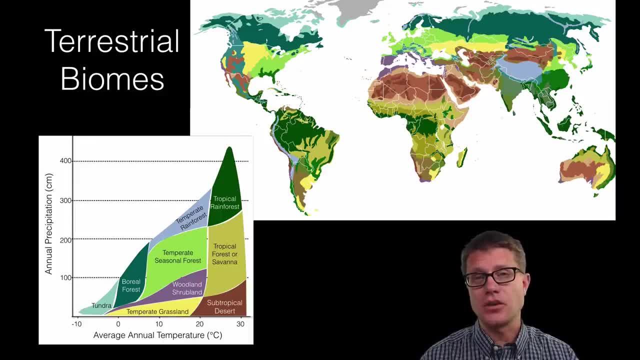 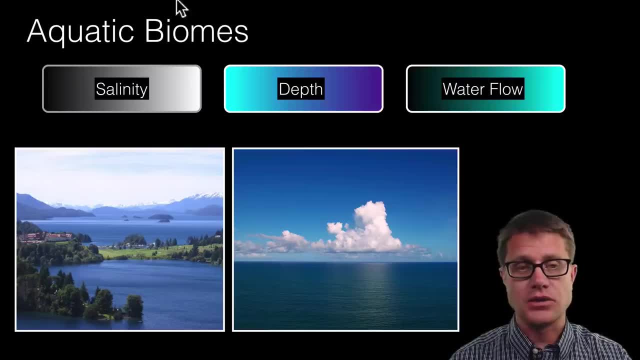 they receive tons and tons of precipitation throughout the year, And so you can see that those are the major biomes. If we start looking at aquatic biomes, it is not temperature and precipitation, because water exists And so it is going to be salinity, the amount of 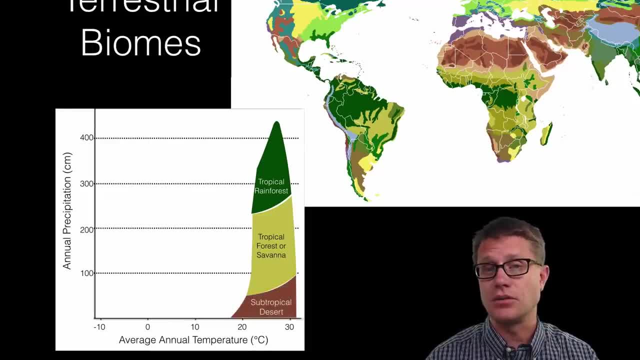 up so we have even less precipitation, then we are going to get into a subtropical desert, And you can see those at this latitude and at this latitude right here. If we keep going across from Africa, though, let's go up here- we are then going to get into a subtropical. 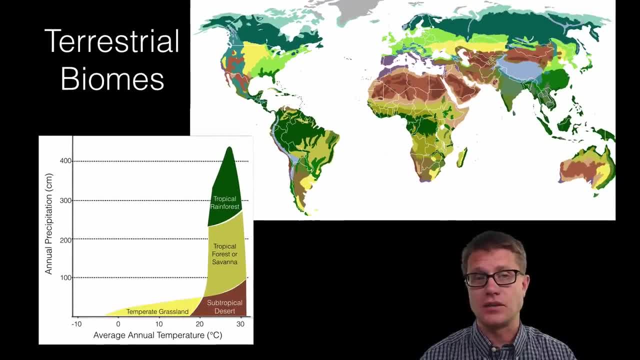 desert And you can see those at this latitude and at this latitude right here. If we keep going to have temperate grassland, sometimes we have temperate deserts. You could see that we have a lot of those in the Midwest of the United States. If we keep going, then we are. 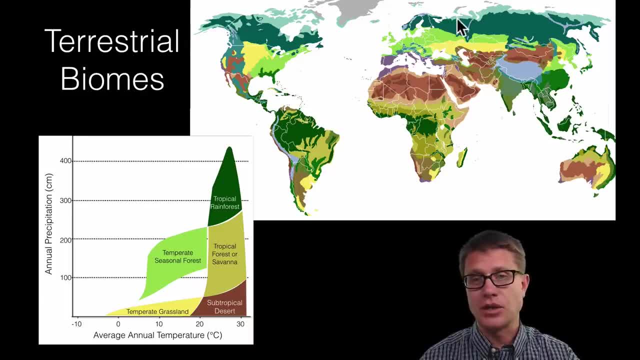 going to get to temperate seasonal forests. If we keep going, then we go to the boreal or northern forests And then we eventually get to the tundra. So these are the major biomes. We could fill in a couple of other ones. So right here in the Mediterranean we 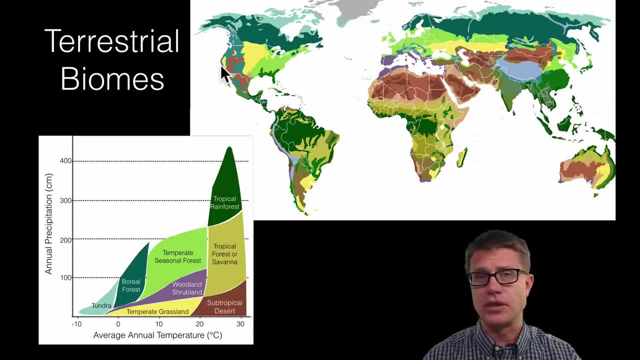 are going to have woodland shrublands. We would have that over in California as well- And then, if we go up here, we will have these temperate rainforests. where it is cooler. they receive tons and tons of precipitation throughout the year, And so you can see those. 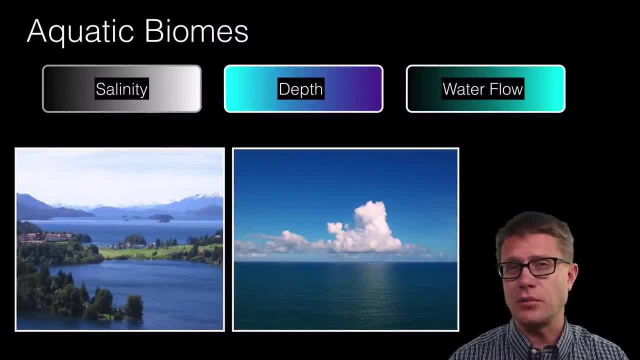 are the major biomes. If we start looking at aquatic biomes, it is not temperature and precipitation, because water exists, And so it is going to be salinity, the amount of salt, the depth within that water, and then the flow of the water. And so the first way, 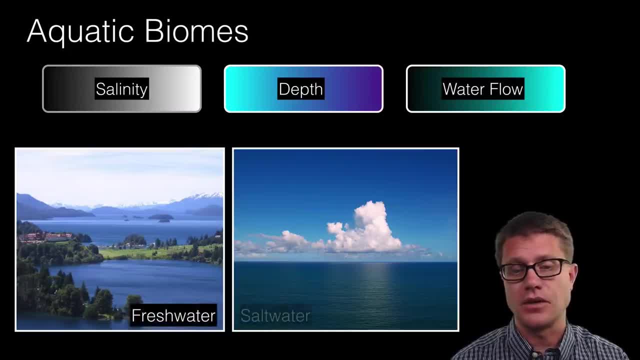 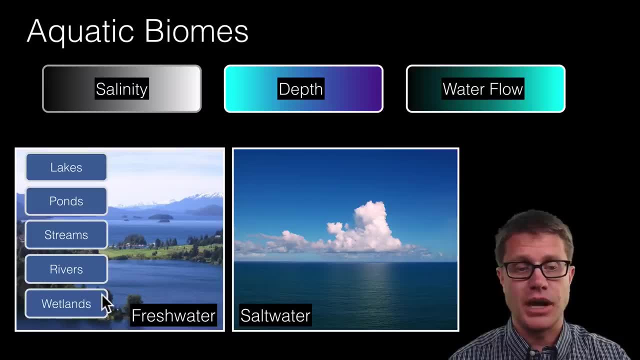 to divide the aquatic biomes is to those that are freshwater and those that are going to be saltwater. If we look at those that are freshwater, you are probably familiar with almost all of these Wetlands are areas where we are going to have water for a large portion. 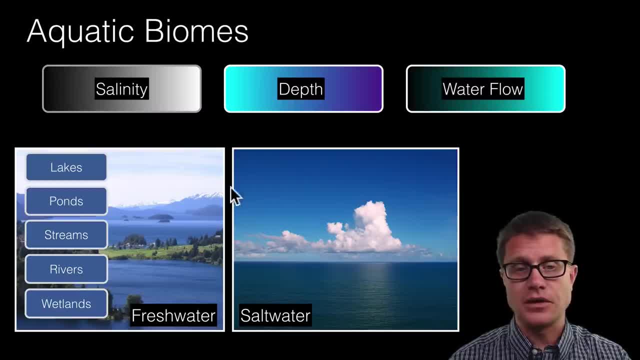 of the year, but we still have vegetation in that area. We could move from there to areas that kind of are in the boundary between fresh and saltwater, So a salt marsh is going to be an area where we have water flowing in, So we can have a mix of freshwater and 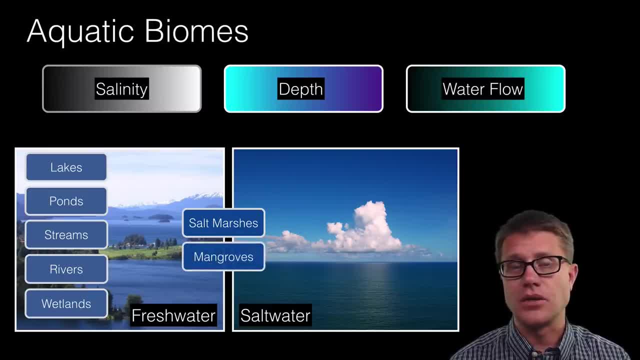 saltwater Estuaries are like this, Or we could have mangroves. Those are areas. mangrove is kind of based on a tree that can grow in saltwater, And those are important as a border between marine and terrestrial systems. And then, as we move out to the ocean itself, we 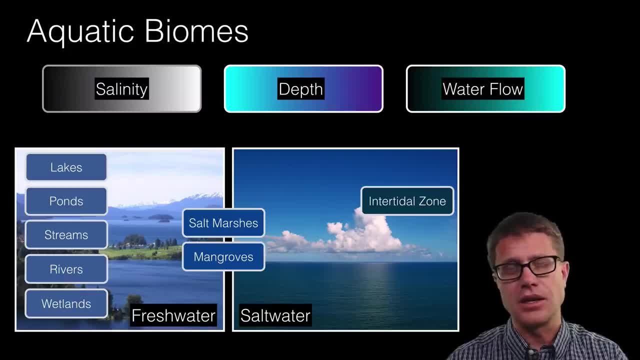 have intertidal zones, So that is going to be when the tide comes in and out. That is that thin area along the coast, Coral reefs you are probably familiar with, and open oceans. Open oceans are really not a super productive ecosystem out in the middle of the ocean. 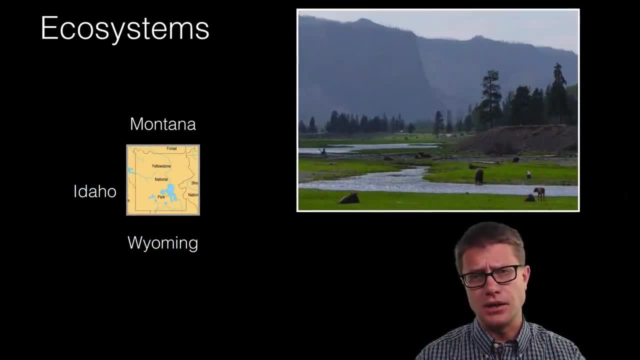 Only near the top, where we get a certain amount of light. So now we are going to go from biome to ecosystem. So this is going to be a smaller area, but it is still really big. One of the most famous ones in the world is the greater Yellowstone ecosystem. It is really just north. 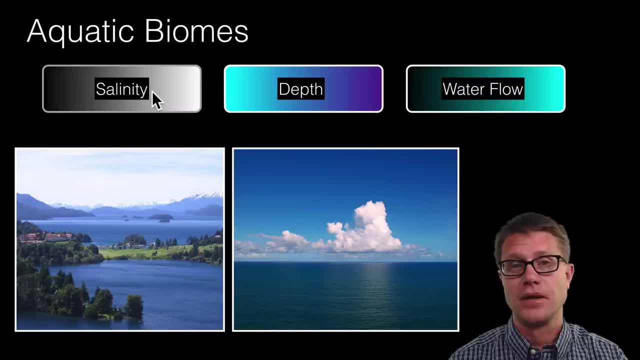 salt, the depth within that water and then the flow of the water, And so the first way to divide the aquatic biomes is to those that are freshwater and those that are going to be saltwater. If we look at those that are freshwater, you are probably familiar with- 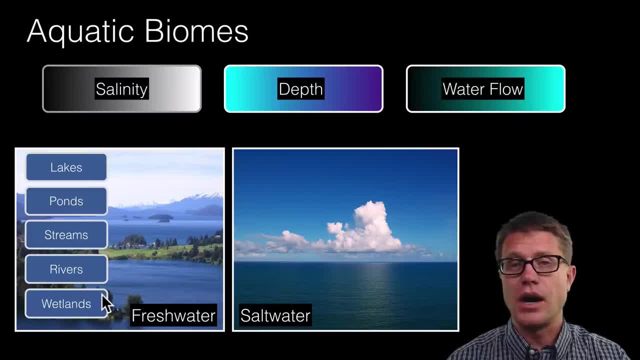 almost all of these Wetlands are areas where we are going to have water for a large portion of the year, but we still have vegetation in that area. We could move from there to areas that kind of are in the boundary between fresh and saltwater, So a salt marsh is going. 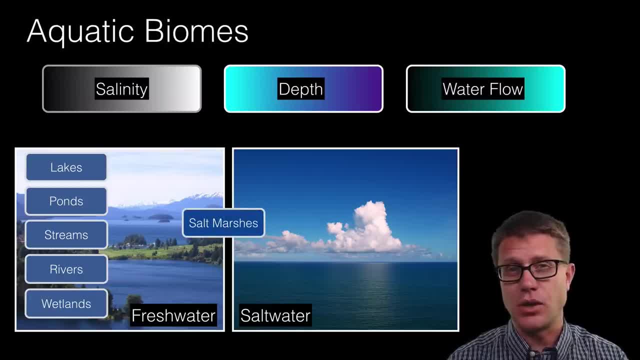 to be an area where we have water flowing in So we can have a mix of freshwater and saltwater. Estuaries are like this, Or we could have mangroves. Those are areas. mangrove is kind of based on a tree that can grow in saltwater And those are important as a border. 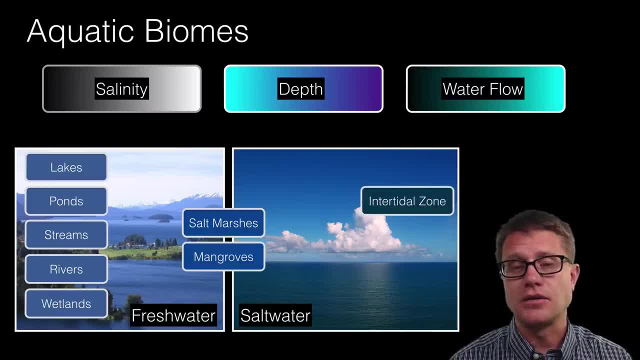 between marine and terrestrial systems And then as we move out to the ocean itself, we have intertidal zones. So that is going to be, when the tide comes in and out, That thin area along the coast- Coral reefs you are probably familiar with. You are probably familiar. 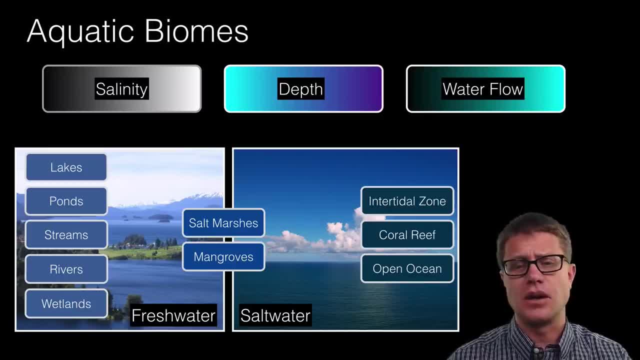 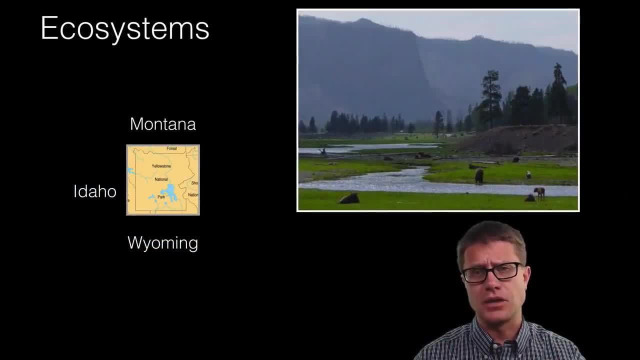 with an open ocean. Open oceans are really not a super productive ecosystem, out in the middle of the ocean, Only near the top, where we get a certain amount of light. So now we are going to go from biome to ecosystem. So this is going to be a smaller area, but it. 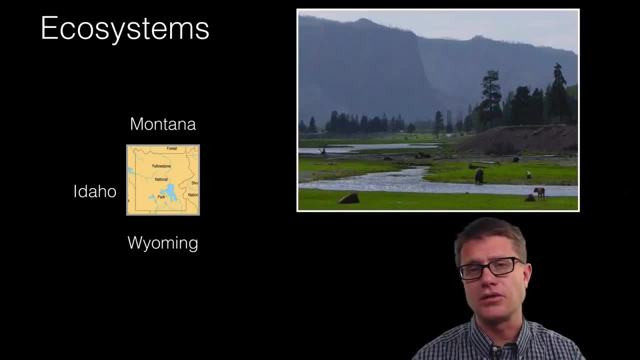 is still really big. One of the most famous ones in the world is the greater Yellowstone ecosystem. It is really just north of me, I live right here- And so it is bordered by Montana, Idaho, Wyoming and Wyoming. But it is not just Yellowstone National Park that. 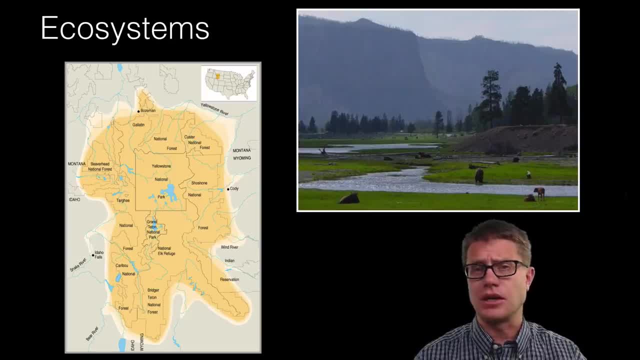 makes up the ecosystem. It is going to be this whole area around it which is going to contain the national park. But it is going to contain the national park, But it is going to also include national forest and private land as well. It is a really large area. It. 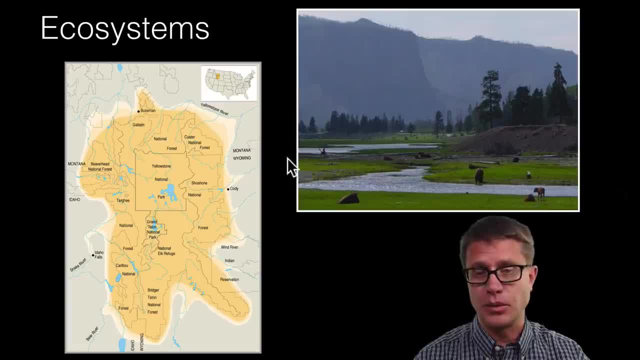 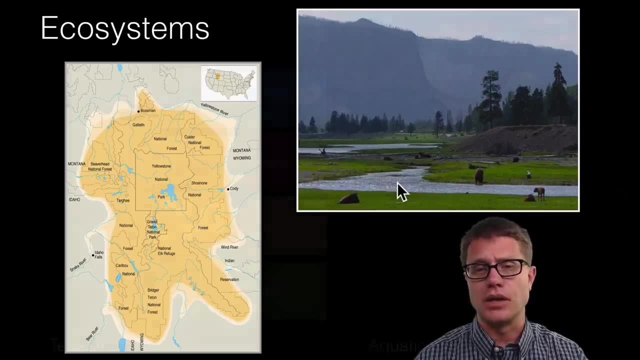 also includes all the abiotic or non-living materials. So, for example, the temperature, the pH of this water, the flow of that water are all considered when we are thinking about the ecosystem. Now let's go to the parts of the ecosystem. So everything is built on these. 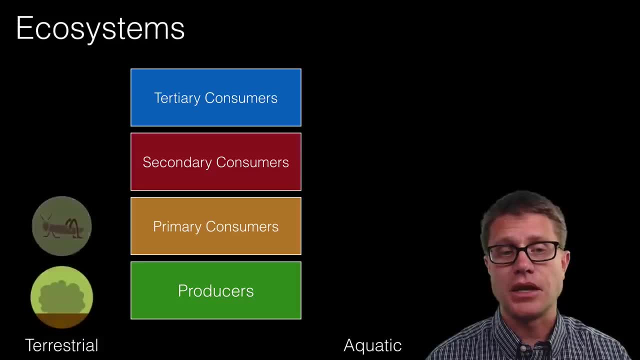 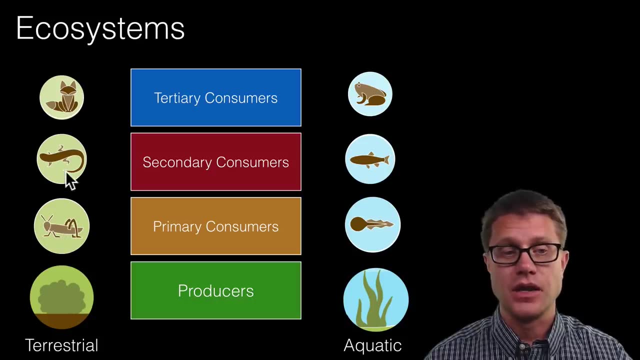 producers And so those things that do photosynthesis. If we look at a terrestrial versus an aquatic, we are going to find the same kind of transition. We have got the plants at the bottom, We have got the herbivores, Then we have carnivores and carnivores on top. So we have these different. 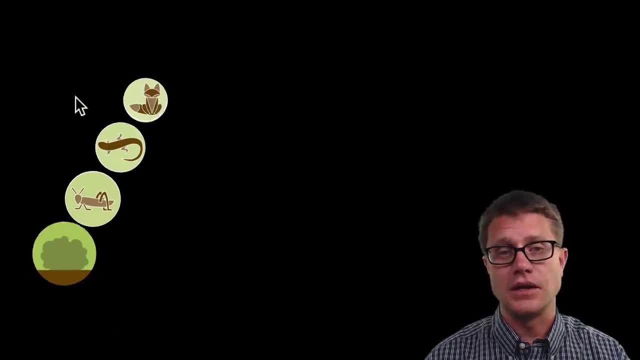 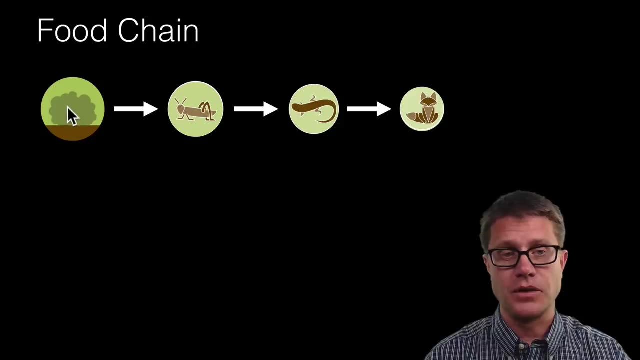 levels of consumers as we move up. They are organized in what is called a food chain And the arrow is going to show where the energy is going or where the food is going. So food goes from the plant to the insect itself. Students sometimes confuse which way the arrows. 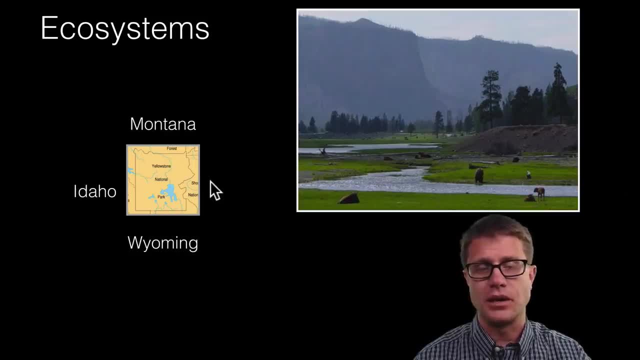 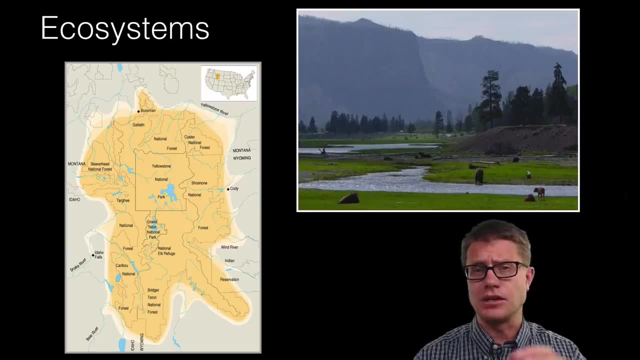 of me. I live right here, And so it is bordered by Montana, Idaho, Wyoming and Wyoming. But it is not just Yellowstone National Park that makes up the ecosystem. It is going to be this whole area around it which is going to contain the national park, but also national 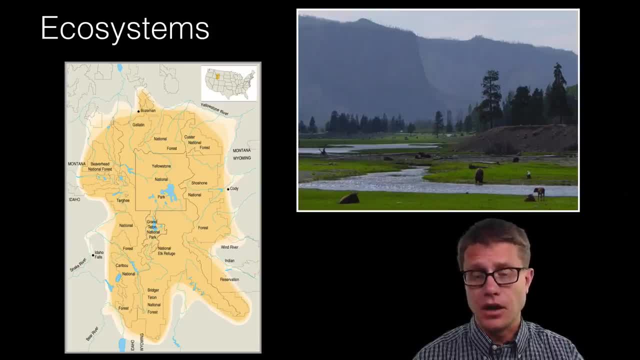 forest and private land as well. It is a really large area. It also includes all the abiotic or non-living materials. So, for example, the temperature, the pH of this water, the flow of that water, are all considered when we are thinking about the ecosystem. Now let's go. 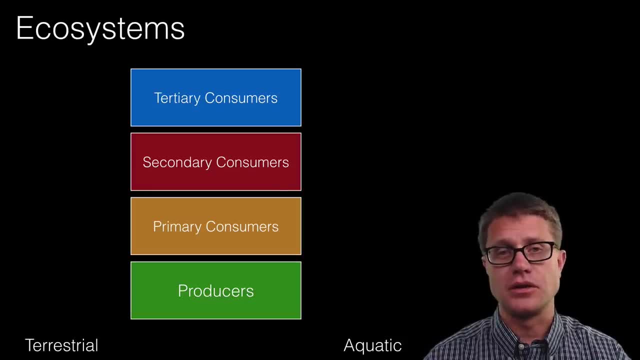 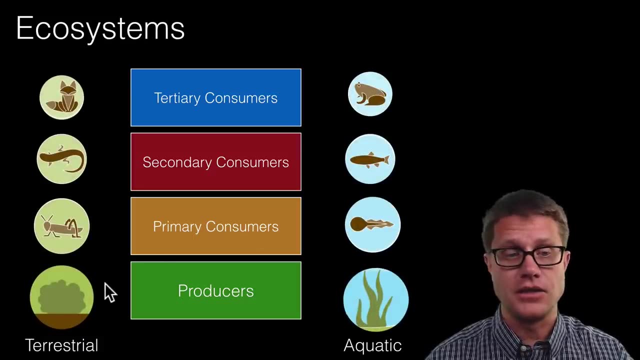 to the parts of the ecosystem. So everything is built on these producers And so those things that do photosynthesis. If we look at a terrestrial versus an aquatic ecosystem, we are going to find the same kind of transition. We have the plants at the bottom, The herbivores. 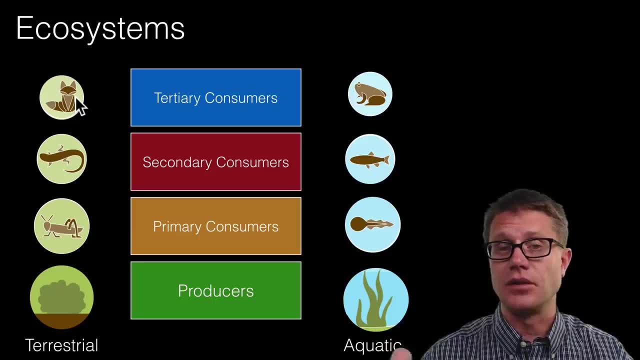 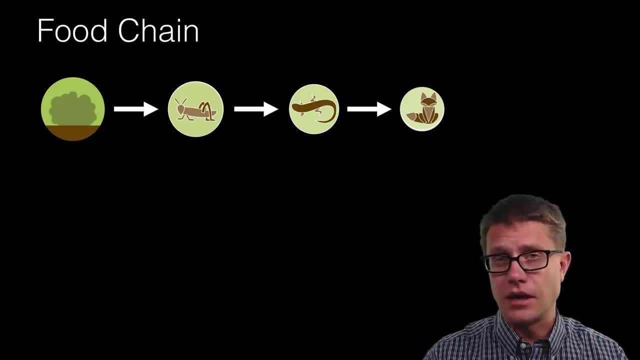 Then we have carnivores and carnivores on top. So we have these different levels of consumers as we move up. They are organized in what is called a food chain And the arrow is going to show where the energy is going or where the food is going. So food goes from the plant. 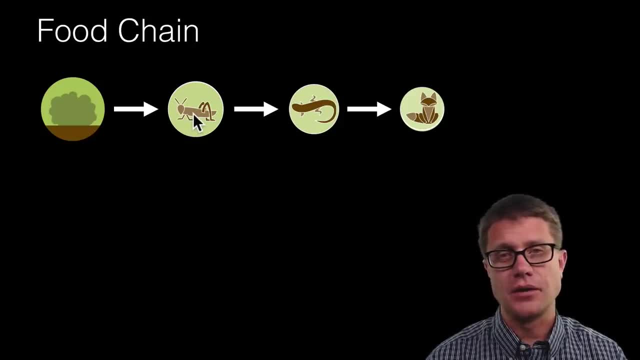 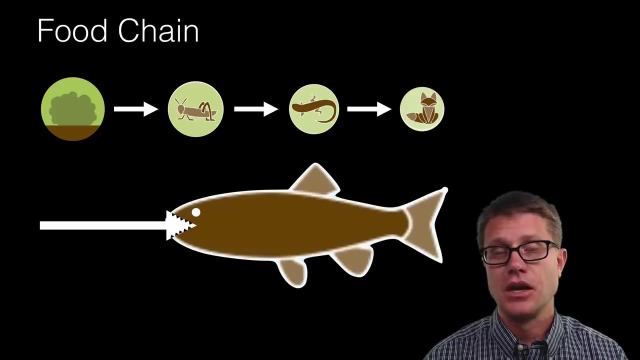 to the insect itself. Students sometimes confuse which way the arrows go, And here is an easy way to remember that. So just think of the arrow as the mouth of what is eating it. So the mouth of a fish. We know that the arrow always goes from the food to what is eating. 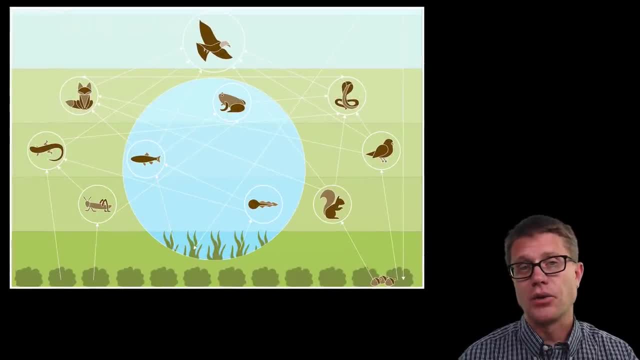 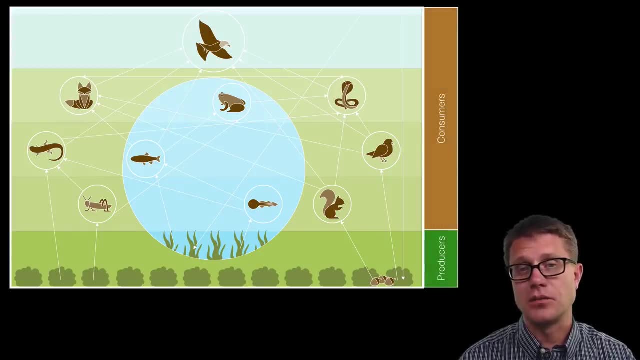 it, Or the organism to what eats that organism. If we organize all the food chains in an area, then we have a food web And so it is going to have producers on the bottom And then it is going to have the consumers above that- Different levels of consumers, If you look. 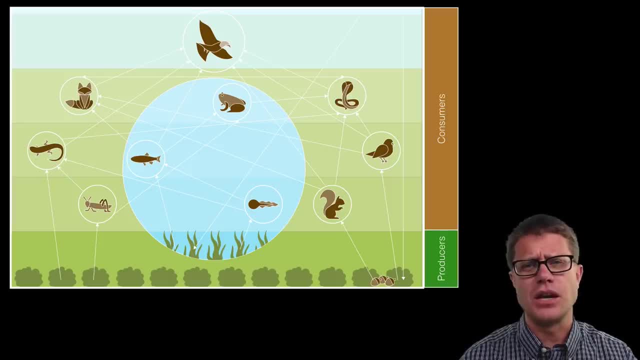 we have got aquatic and terrestrial, all mixing in. Some terms that you may be familiar with are herbivore. Herbivore is going to be something that just eats plants. We have got carnivore, Something that just eats other plants. We have got herbivores, We have got carnivores. 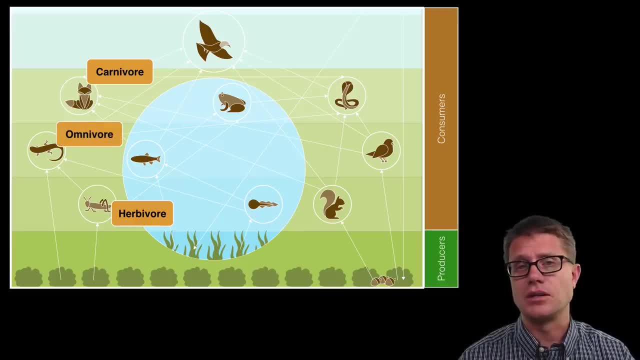 Other living things, But we also have an omnivore. That is going to be something that eats plants and other living things. Keystone species, remember, is going to be a species that keeps everything kind of in check in that ecosystem, And I am really leaving off. 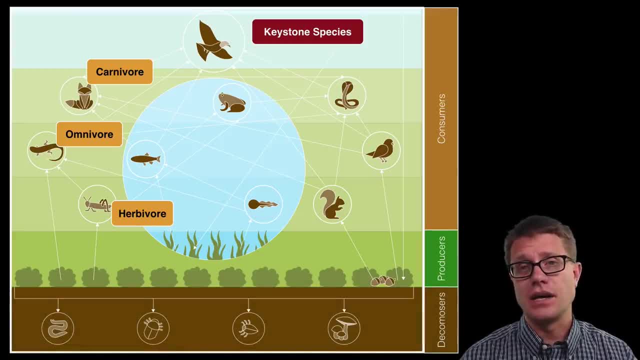 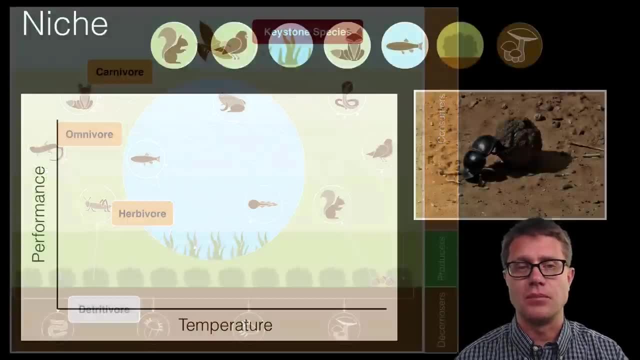 a bunch, which is going to be all the decomposers. So as material dies, we have to recycle that. So that is going to be decomposers. An example are detritivores that can eat large bulk amounts of dead material. What is the niche? Now we are at the level of an individual, So a niche. 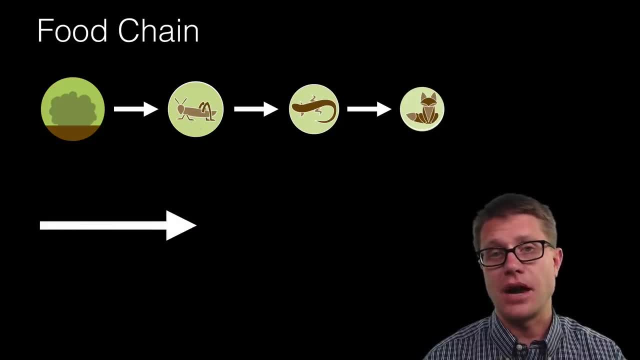 go. And here is an easy way to remember that. So just think of the arrow as the mouth of what is eating it. So if this is the mouth of a fish, we know that the arrow always goes from the food to the food. So if this is the mouth of a fish, we know that the arrow always 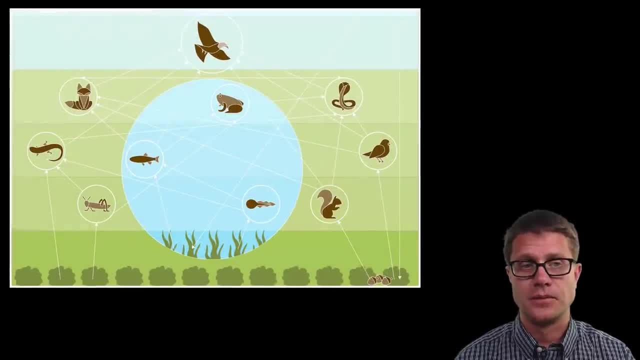 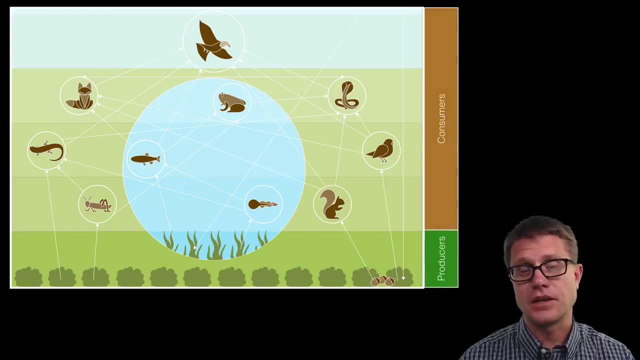 goes from the food to what is eating it, Or the organism to what eats that organism. If we organize all the food chains in an area, then we have a food web, And so it is going to have producers on the bottom And then it is going to have the consumers above that. 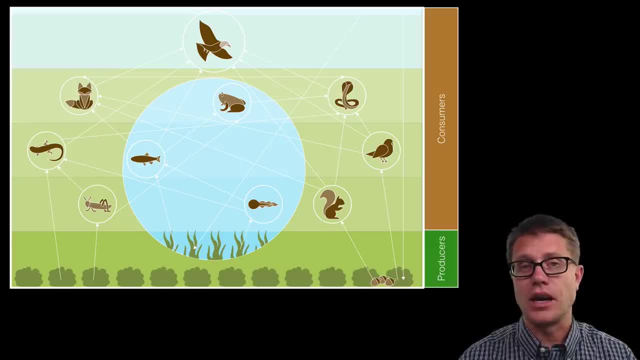 Different levels of consumers. If you look, we have got aquatic and terrestrial all mixing in. Some terms that you may be familiar with are herbivore. Herbivore is going to be something that just eats plants. We have got carnivore, Something that just eats other living things. 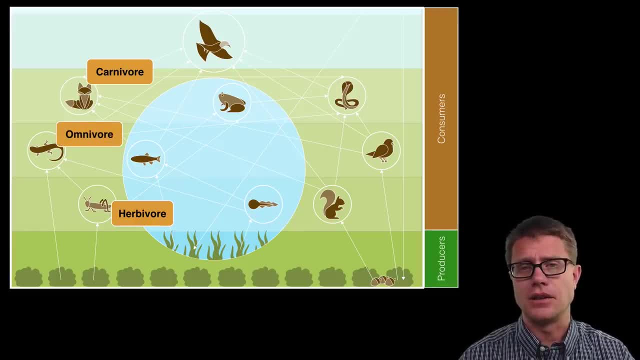 But we also have an omnivore- That is going to be something that just eats plants. We have got carnivore- That is going to be something that just eats other living things. But we have got carnivore- That is going to be something that just eats plants and other living things. 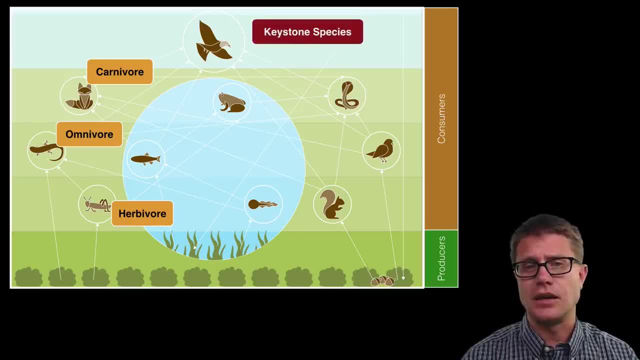 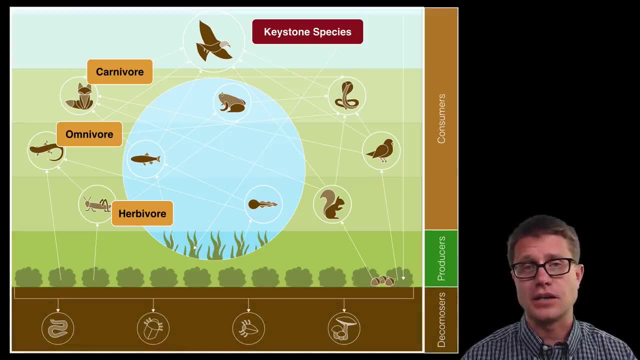 Keystone species, remember, is going to be a species that keeps everything kind of in check in that ecosystem And I am really leaving off a bunch which is going to be all the decomposers. So, as material dies, we have to recycle that. So that is going to be decomposers. An example: 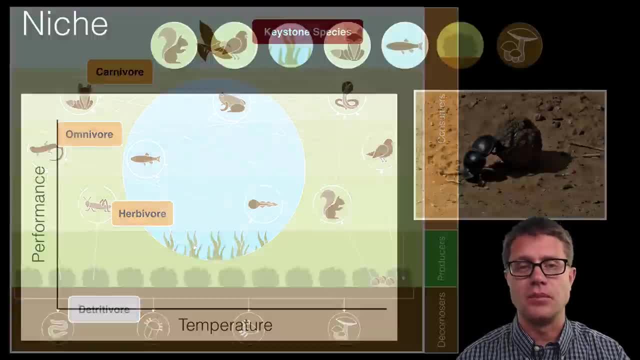 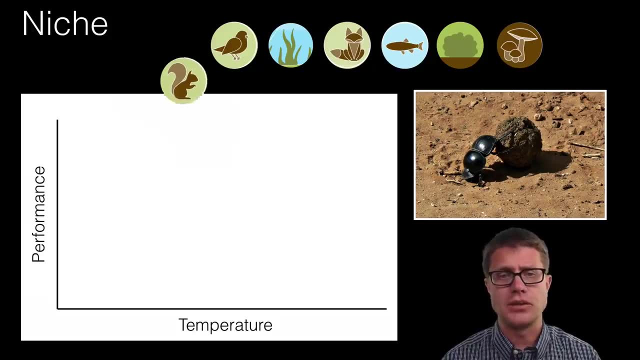 are detritivores that can eat large bulk amounts of dead material. What is the niche? Now we are at the level of an individual, So a niche you can think of as like the job of an individual. So if we take this squirrel and say, how does the squirrel perform over different temperatures? 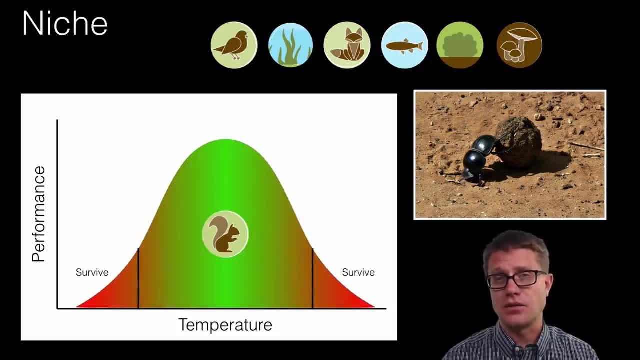 Well, we are going to get a distribution like that. There are going to be areas where it can survive Outside. that would be areas where it dies If it is too cold or if it is too hot. As we move closer to the middle, we get areas where it can survive and grow. And finally, 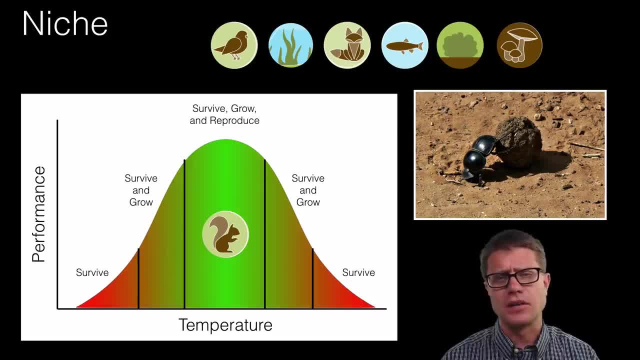 where it can survive, grow and reproduce, And so the environment has a lot to do with the niche, But also what we are using as a food source. So this dung beetle, for example, exploits a niche by taking dung, rolling it up and using that as an eventual food source. 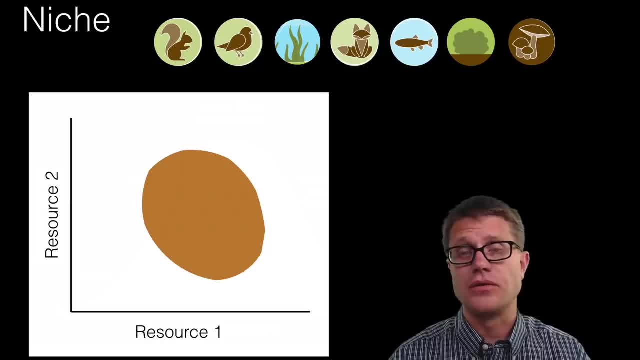 What else determines it, then? not only the environment, but the resources, the food that you need or the space you need to live in, And so we can represent that on this graph, as here is the two resources I need, and that is going to be my fundamental niche. That is where this squirrel could live. 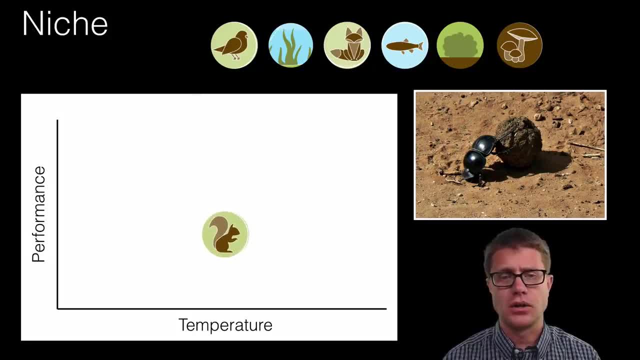 you can think of as like the job of an individual. Take a squirrel and say: how does the squirrel perform over different temperatures? Well, we are going to get a distribution like that. There are going to be areas where it can survive. Outside that would be areas where it dies If it is too cold or if it is too hot, As 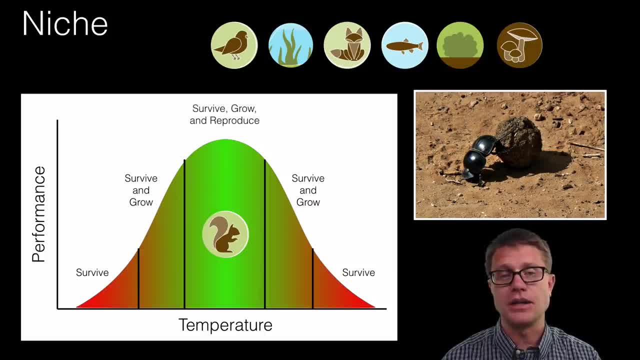 we move closer to the middle, we get areas where it can survive and grow And finally where it can survive, grow and reproduce, And so the environment has a lot to do with the niche, But also what we are using as a food source, So this dung beetle, for example. 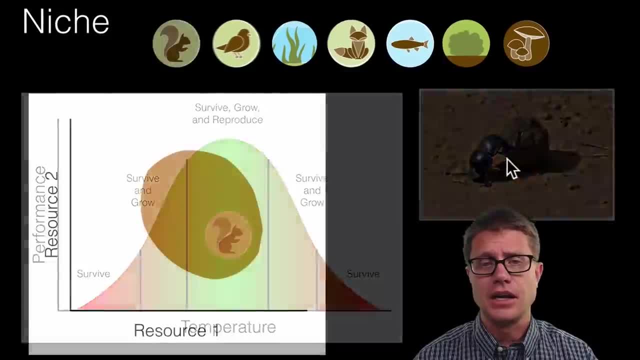 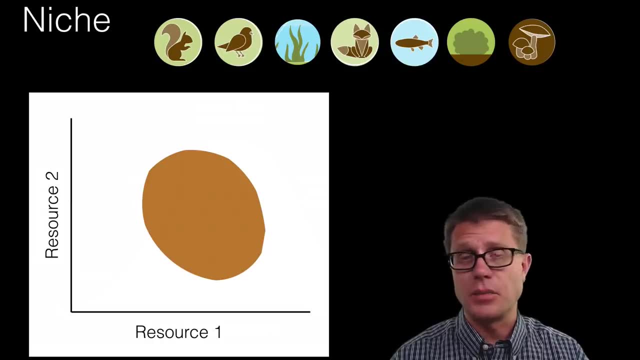 exploits a niche by taking dung, rolling it up and using that as an eventual food source. What else determines it, then? Not only the environment, but the resources, The food that you need or the space that you need to live in, And so we can represent that on this graph. 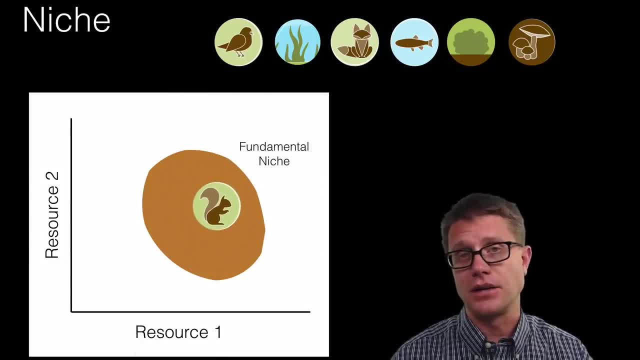 as here are the two resources I need and that is going to be my fundamental niche. That is where this squirrel could live. Now what you will find is that it actually does not fit that way. You have what is called a realized niche where it could live in all that areas. but it only lives in the small area And the realized niche is a niche that is completely 피 ihnne. It is not in the large area. In fact, it lives in the small area, And the realized niche is a niche that is actually not in the large area. There is a niche that is actually an 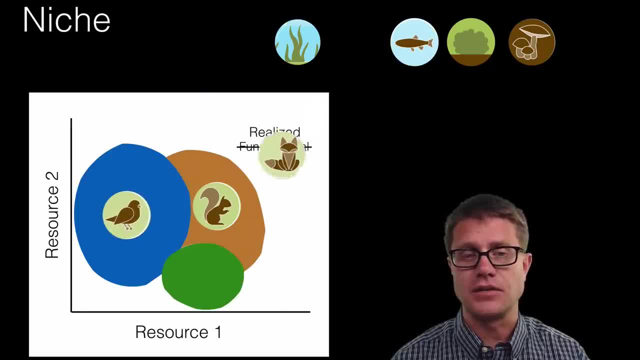 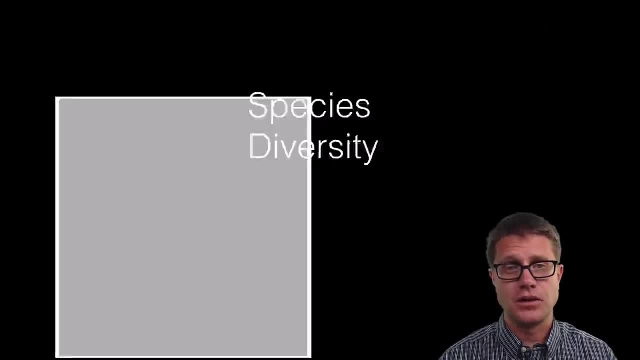 area, And the reason why you are probably guessing is that there are other niches outside, that There is competition going on. Species diversity is actually good. It is good to have all these different species. So let me use this model to show you how that works. 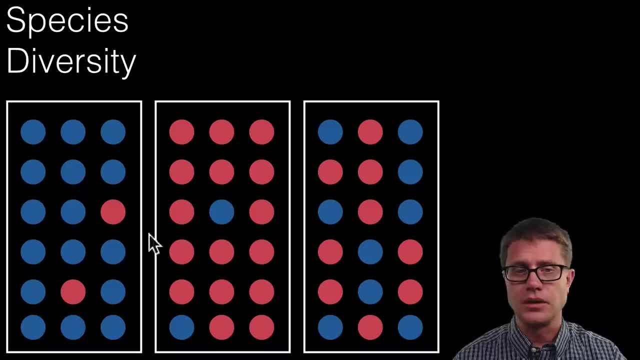 Imagine we have species that are just cold tolerant, They love the cold, Warm tolerant, They love the heat Or a nice diverse mix of the two. And so let's say we apply some cold weather. What happens? All those that are not cold tolerant die. You can see the. 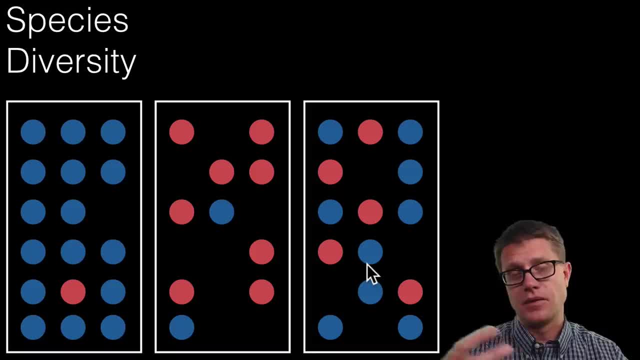 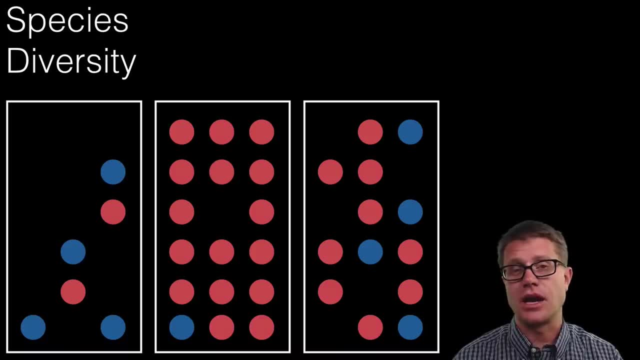 warm, tolerant, are going to be most affected. You are going to see the diverse species in the middle And the cold ones are doing fine. But let's say we change it up now And it is really hot, Then we are going to have this impact. And so, right here, by having a diverse 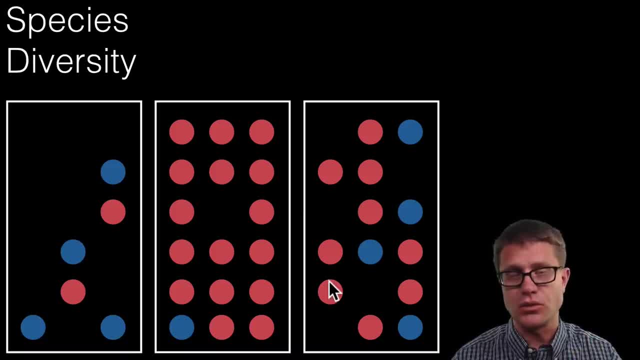 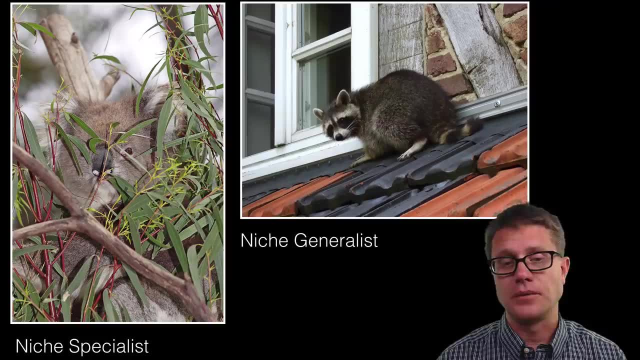 population. this does not have to deal just with temperature, but it can be resources you are feeding on. The more species we have, the healthier that ecosystem is going to be. That even applies at the individual level. So a raccoon is what is called a niche generalist. 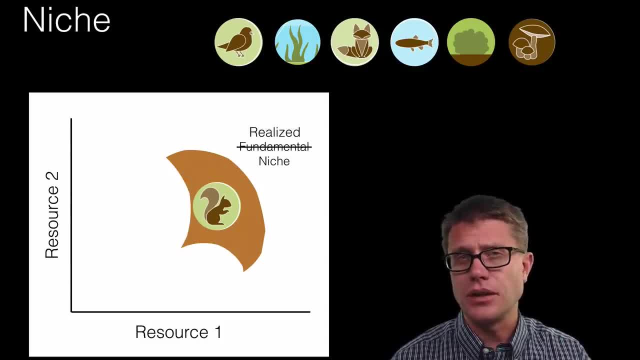 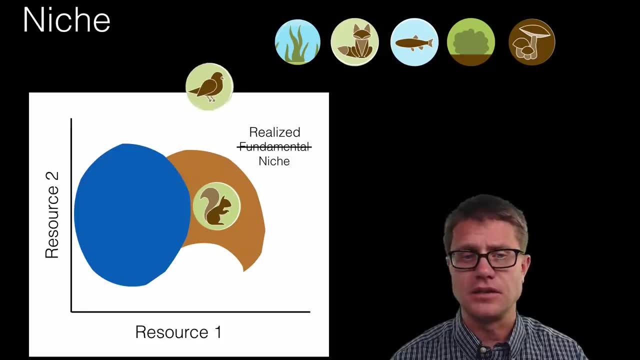 Now what you will find is that it actually does not fit that way. You have what is called a realized niche, where it could live in all that areas, but it only lives in this small area, And the reason why you are probably guessing is that there are other niches outside. 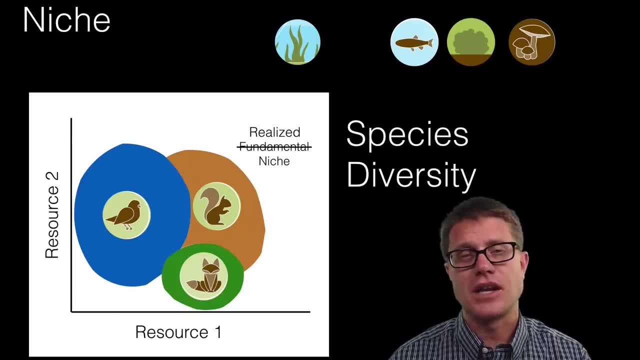 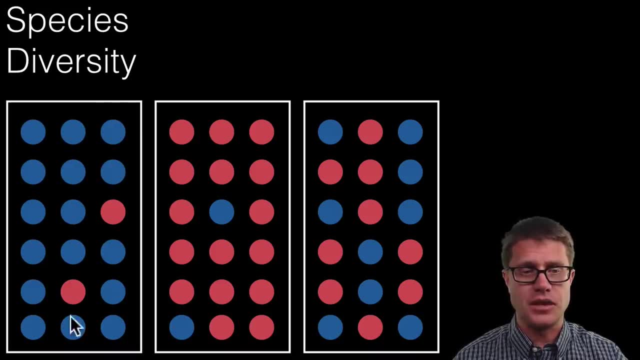 that There is competition going on. Species diversity is actually good. It is good to have all of these different species. So let me use this model to show you how that works. Imagine we have species that are just cold tolerant. They love the cold, Warm tolerant. 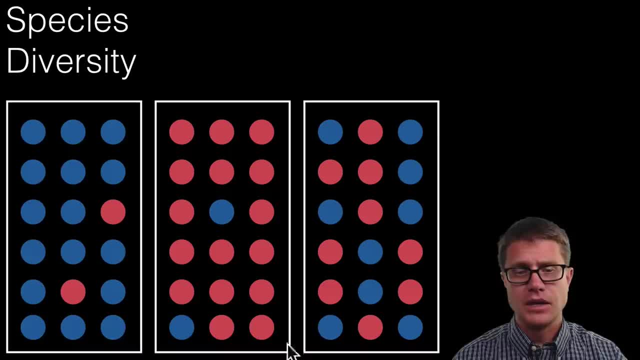 They love the heat Or a nice diverse mix of the two. And so let's say we apply some cold weather. What happens? All those that are not cold tolerant die. You can see the warm tolerant are going to be most affected. You are going to see the diverse species that 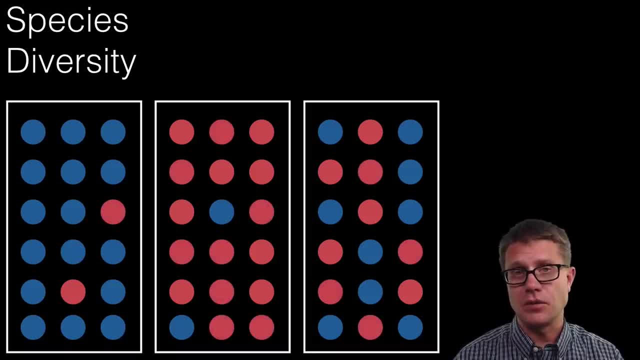 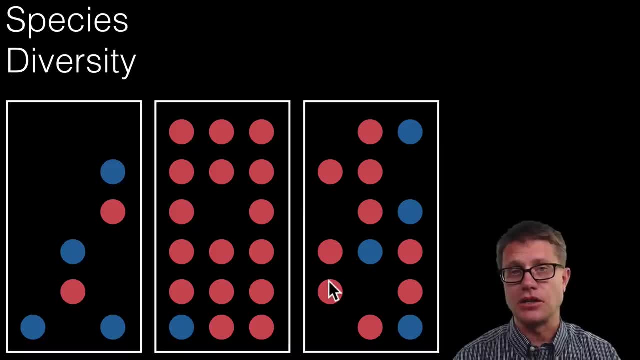 are in the middle And the cold ones are doing fine. But let's say we change it up now And it is really hot. Then we are going to have this impact. And so, right here, by having a diverse population. this does not have to deal just with temperature, but it can be. 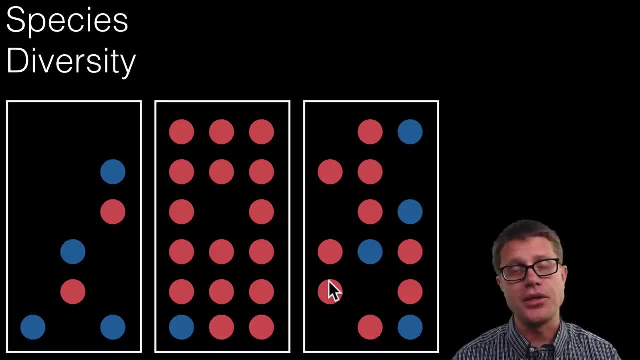 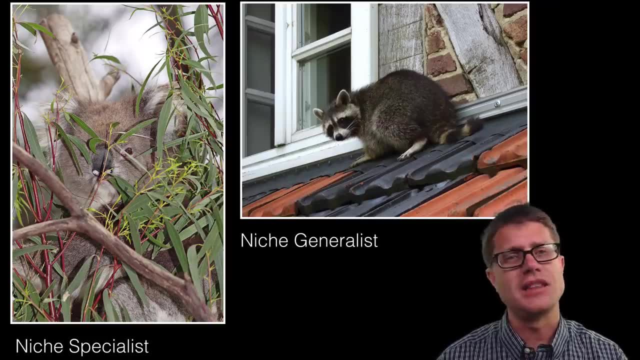 resources you are feeding on. The more species we have, the healthier that ecosystem is going to be. That even applies at the individual level. So a raccoon is what is called a niche generalist. It can eat lots of different food resources. It can live in lots of different. 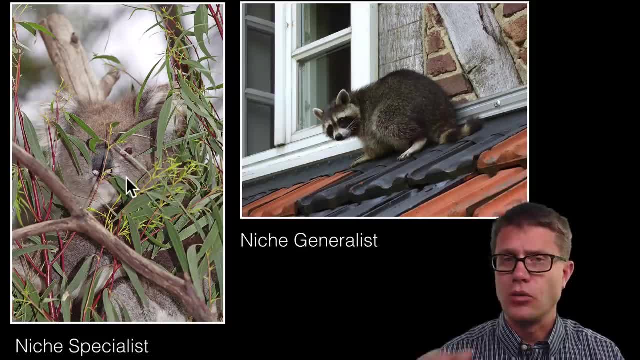 areas, Whereas a koala can only eat eucalyptus leaves. So that is what we are going to do: We are going to change it up. We are going to change it up. Which of these do you think is more susceptible to change in that environment? 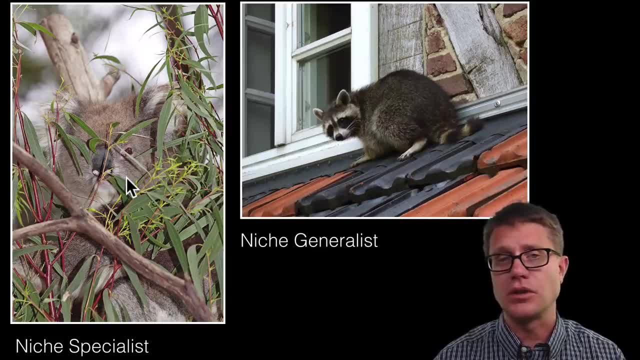 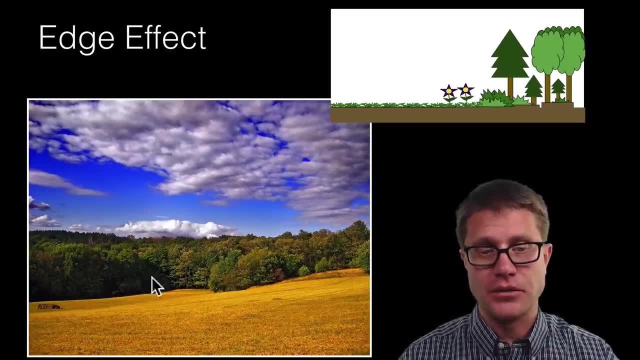 Definitely going to be the koala, Since it is only feeding on one thing. if that resource is impacted, it is going to be impacted as well. The edge effect also affects the health of an ecosystem. Edge effect is going to be a boundary between two ecosystems. It actually 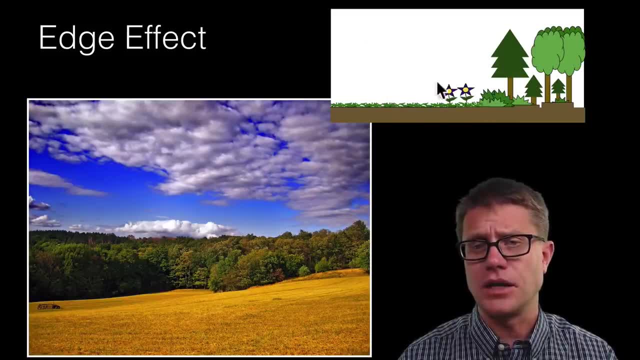 can be a healthy area. So if it develops over a long period of time, what you will get is this transition from here into the forest, And so that is an area where we can actually support more species. The problem is that humans, lots of times 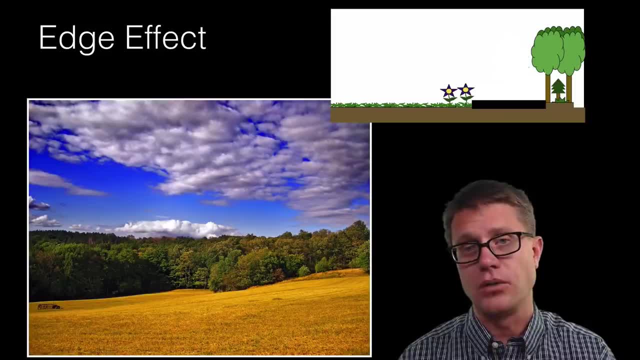 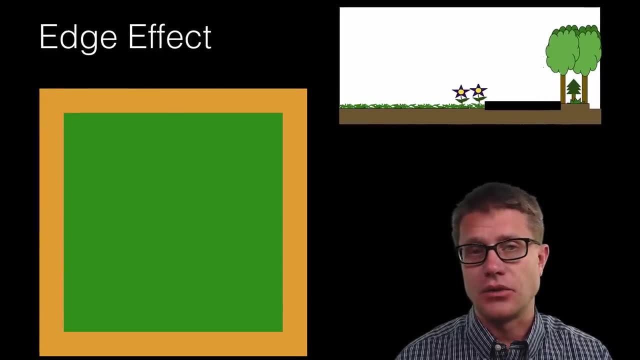 will just create an edge. So we make a trail or we make a road, And now what happens is there is not this natural boundary, And that can damage the health of the ecosystem. The size of the edge is always going to be the same, And so watch what happens when I take.